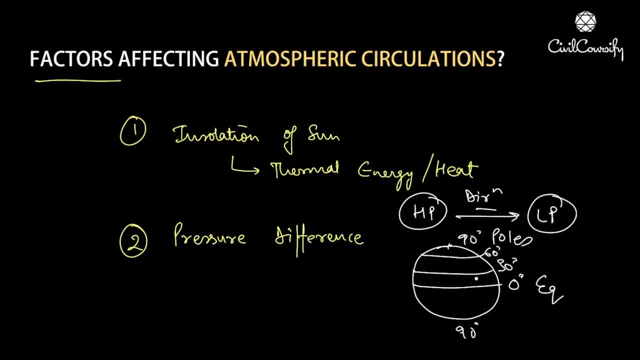 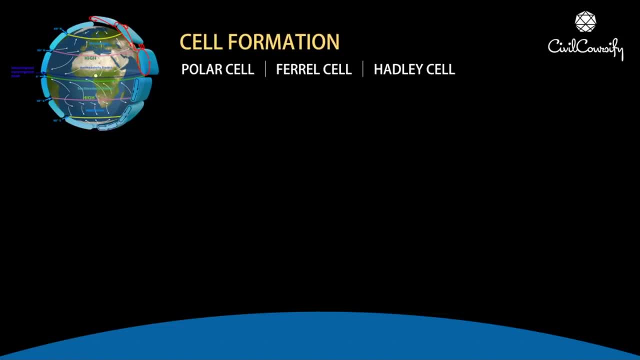 Now we are looking at 0,, 30,, 60, 90 latitudes, because we'll need them to understand the entire concept in this video, Right? so as you can see here that the direction of the wind is different in different latitude belts, 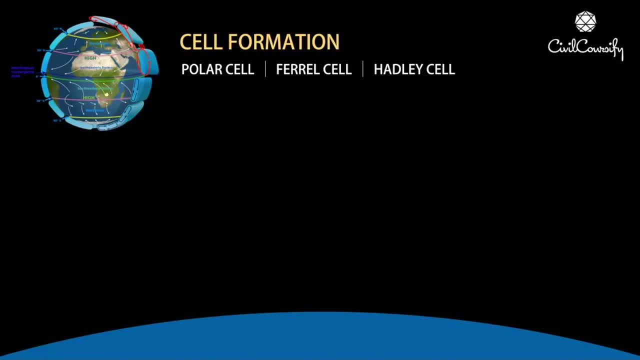 Why is that? We'll see that now. You can also notice that the wind is getting deflected towards the north pole, Towards the left in the Southern Hemisphere and towards the right in the Northern Hemisphere. Why is that? This is because of the Coriolis force, and we have already made a video on the Coriolis effect. 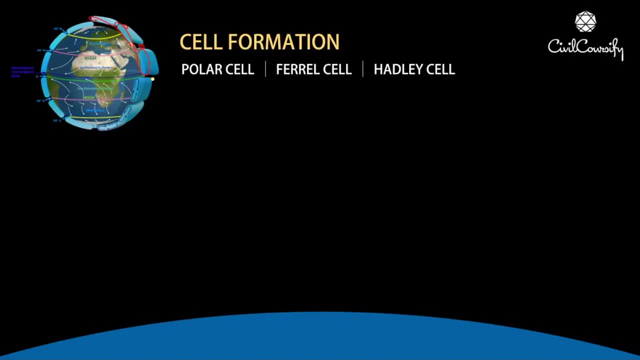 If you haven't seen it yet, you can go to our app and watch it. This video is available there. Right, so we'll start with the equator and we'll move towards the poles- the North Pole in this case- And we'll try and understand the cell formation process. 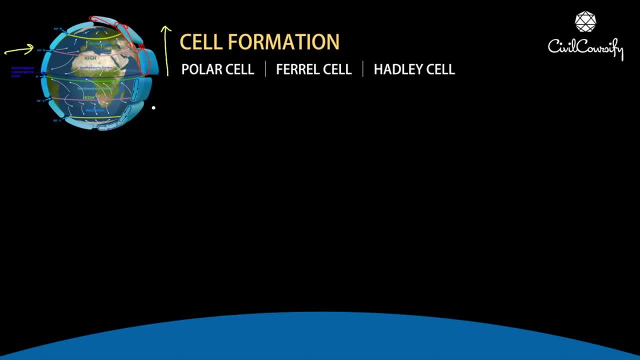 And we'll see the whole process from this direction. This would be our reference, Right? so let us assume this is the 0 degree equator And this is 90 degree latitude And this is 90 degree North Pole. Let us begin with the equator. Now we know that the equator is the hottest. It has the highest average temperature throughout the year. The primary reason for this is that the equator has the highest insolation on an average throughout the year And because of the high temperature. the first thing we should know is that there will be low pressure in this region. 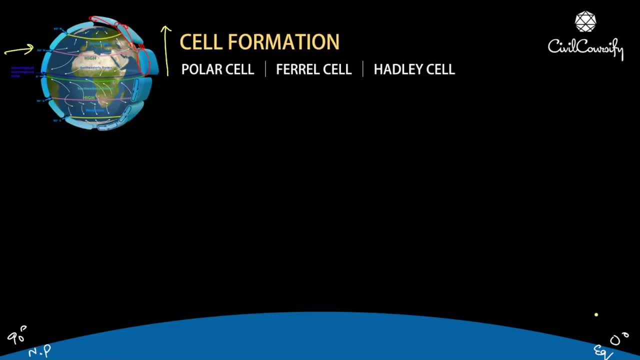 Low pressure occurs where there is a comparatively warm region as compared to the high pressure region. So here there will be low pressure. Now the land will heat up Because of the low pressure. there, the air will rise up, And how long will it rise? 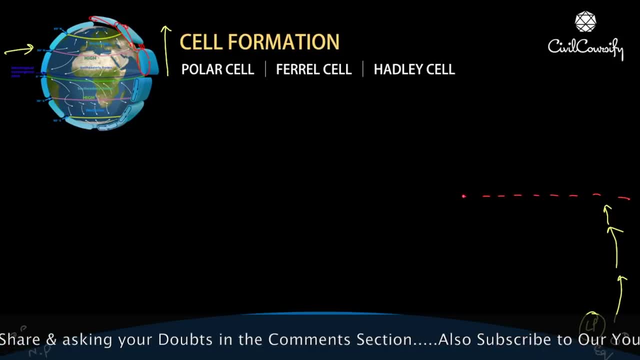 It will rise till the tropopause. Now, what is the tropopause? Tropopause is the junction between the troposphere and the stratosphere. This is the boundary between the troposphere and the stratosphere, which is known as the tropopause. 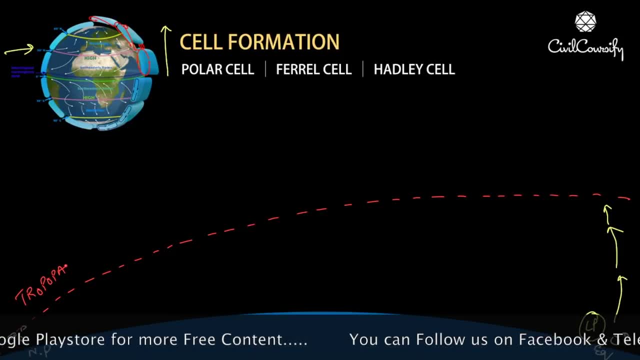 So this is the tropopause. Now the air would remain in the troposphere. It cannot go to the stratosphere, So it will have to stop at the tropopause. Now how will it stop? It will try to diverge at the tropopause. 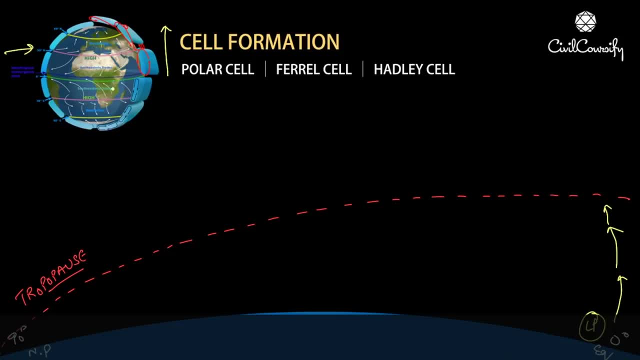 Now, as we have already discussed in the ITCZ video, that the north-easterly trade winds and south-easterly trade winds converge in the ITCZ region and they rise up, So near the equator, basically in the ITCZ region in both cases, when the north-easterly trade winds and south-easterly trade winds converge and rise up, 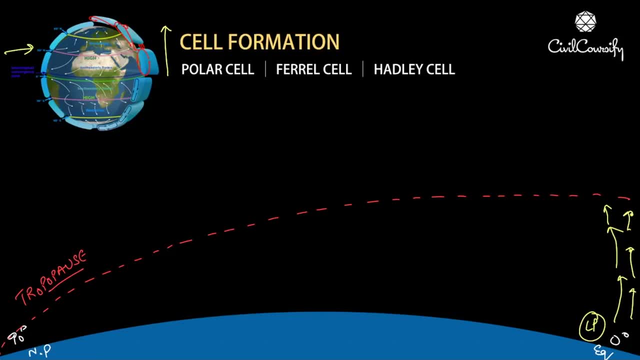 till the tropopause. then they will diverge. Half of the part will go towards the north pole and the other half will diverge towards the south pole. That is why different cells will form in the northern hemisphere and in the southern hemisphere. So when the air rises at the zero-degree equator, and basically at the ITCZ, 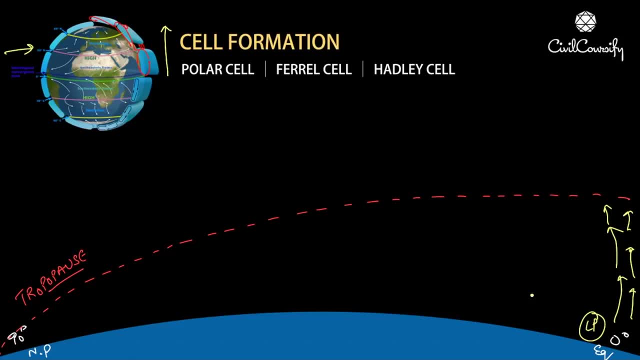 because in the ITCZ video we saw that the ITCZ is the one that produces the most low pressure and here the air will rise up And, after diverging at the tropopause, it will start moving towards the north-easterly trade winds. 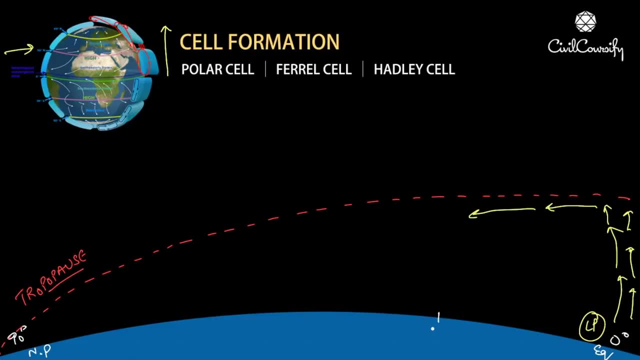 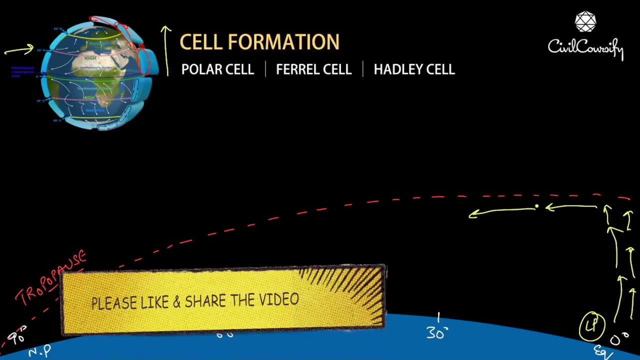 Towards the poles. Now let's say this is 30-degree latitude and this is the 60-degree latitude. Now, as the warm air rises up, diverges and reaches here, it will cool down. And when the air mass cools down it tries to subside. 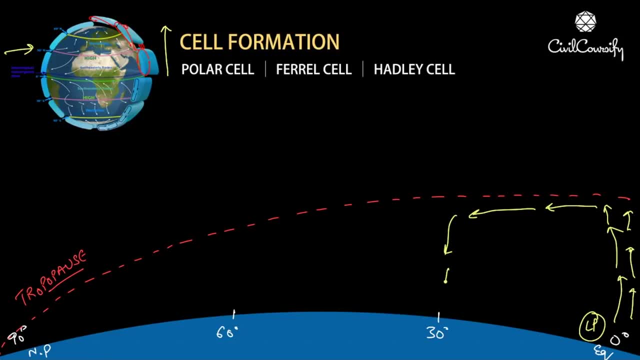 It will subside towards the land. And when the air subsides towards the land mass, it has two parts: Some will go here and some will go there. So let's say now we just look at this direction, Which is this direction? 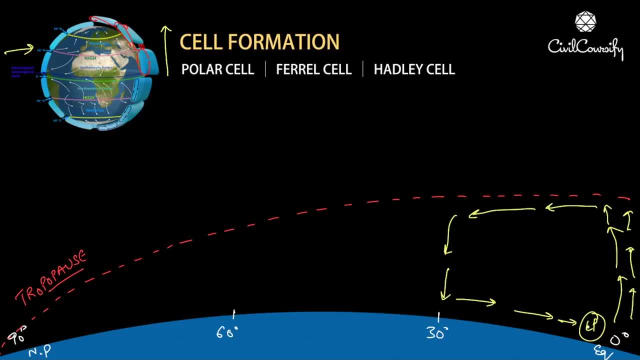 The air is going here towards the equator. This will complete a cycle because after reaching the zero-degree equator it will rise up again, converging with the south-easterly trade winds. So these winds which are moving on the surface of the earth are known as north-easterly trade winds. 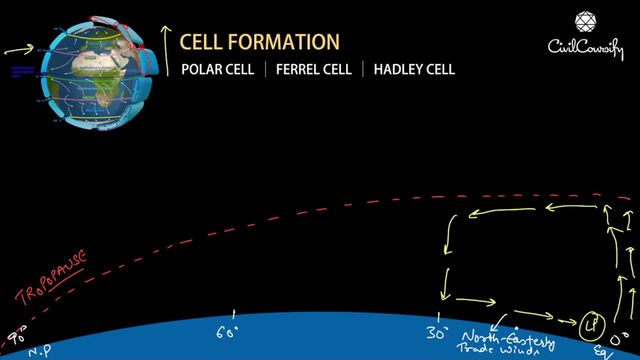 Now these are also known as subtropical easterlies, because they are moving in the subtropical region. Now this complete cell is known as the Headley cell. Now, why is it called the Headley cell? Because this theory was given by George Headley. 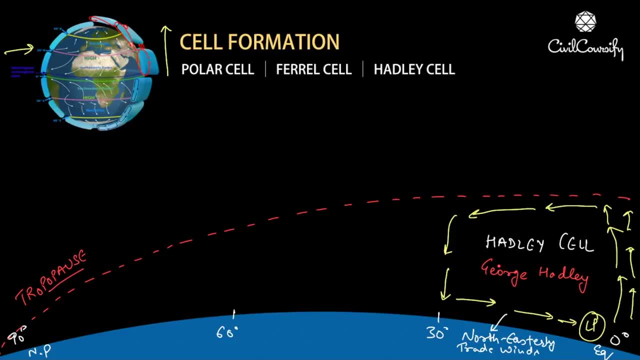 He gave this theory while describing how the trade winds emerge. Now let's come to the polar cell. Now, before we discuss the polar cell, you might have noticed that we have subsided the tropopause towards the north pole. Why is that? The height of the tropopause is the lowest on the north pole and the highest on the equator. 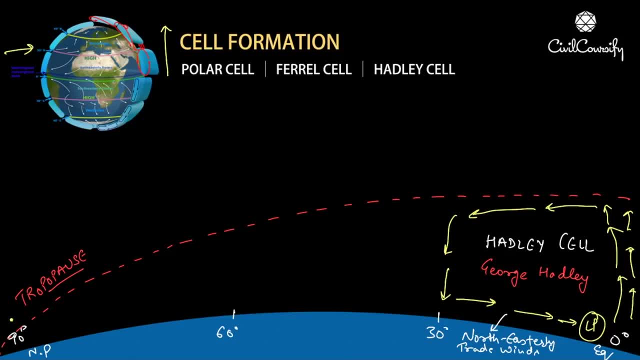 The reason for this is that the air is dense at the north pole. Because of this, the tropopause is at the bottom And if you want to understand it in a very simple way, let's say the temperature of the tropopause, for example, is minus 80 degrees Celsius. Now, to achieve minus 80 degrees Celsius on the equator, you have to go to a very high altitude, Because on the equator, let's say on an average, if the temperature is 30,, 35,, 40 degrees Celsius. then slowly going down to minus 80 degrees. you will have to travel a lot of distance, But on the north pole the temperature is already minus 10,, minus 15,, minus 20 degrees Celsius, And to go to minus 80 degrees you don't have to travel a lot of distance. 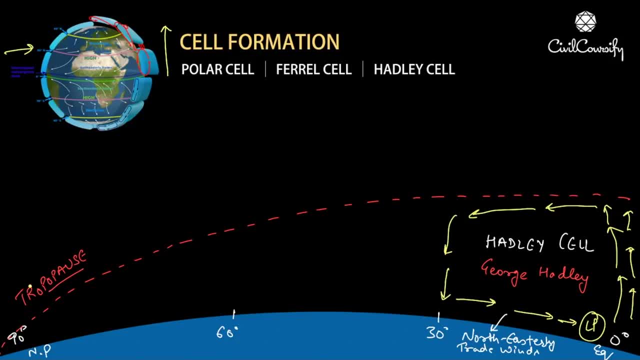 If we talk about the altitude. That is why the tropopause is very low at the poles Right. so we were talking about the polar cell. The first thing we should know is that the temperature on the poles is the lowest. so, due to the very low temperature on the north pole, 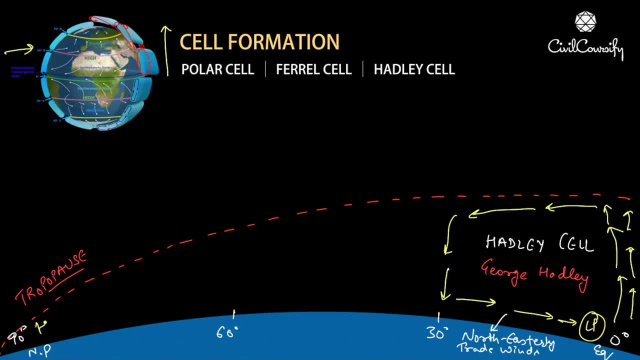 due to the minimum insolation, there will be a high pressure, As we saw that there was a low pressure on the equator because of high insolation, due to the heat up on the land, due to the warm region, similarly, due to the cold region. 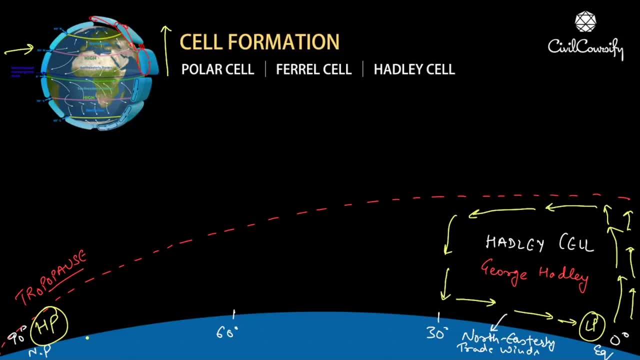 there will be a high pressure at the poles. Now the wind will move towards the low pressure from the high pressure. and when the wind will go towards the equator from the poles, it will reach the 60 degree latitude. and here, comparatively, 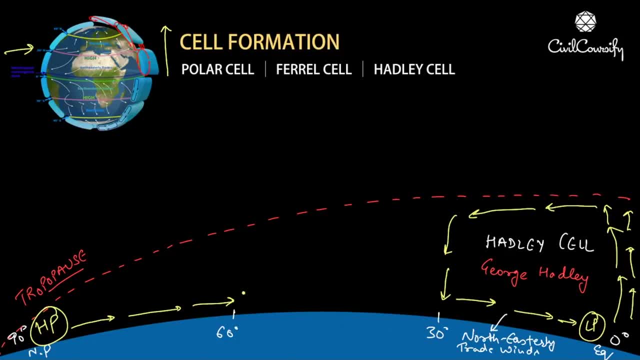 the air in the wind would have warmed up, And after it gets a little warm it will try to rise up. Now, where will it rise? It will rise till the tropopause, because the wind cannot go above the tropopause, the air mass cannot go. 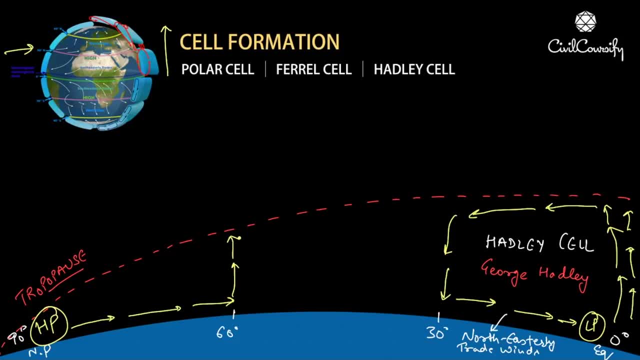 And after it goes here it will try to diverge, as it did in this case, And it will diverge a little bit here, a little bit here. We are seeing only this part now, So if we see it will go in this direction. 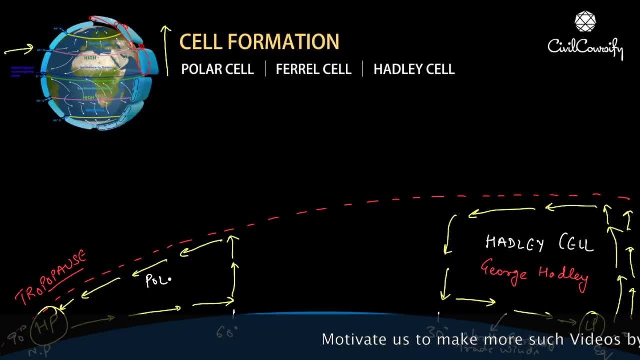 and this is the first cycle. This is what we call the polar cell, And this type of wind on the surface, as you can see here, are known as the polar easterlies. Now we have seen the headly cell and now the polar cell. 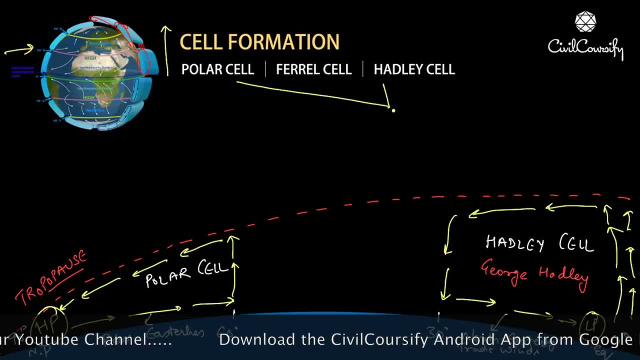 Now you must know that the polar cell and the headly cell are thermal cells, because they are formed due to the insulation of the sun, and this is leading to the pressure difference Where the ferrule cell is. this is a mechanical cell. 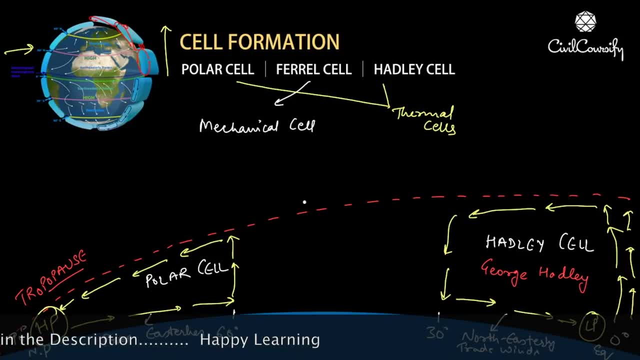 A mechanical cell means that it is being formed because of the void that is being created by these thermal cells. Now a headly cell, a polar cell. the gap between these two cells will form a mechanical cell, which is known as the ferrule cell. 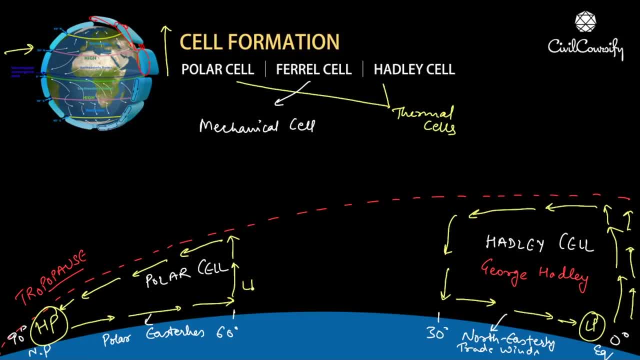 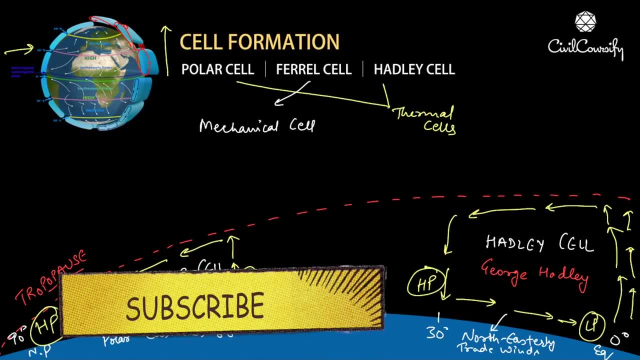 Now, here air rises, so here comparative low pressure was formed As compared to the poles, and here air subsided, so a comparative high pressure was formed as compared to the equator. So now what will be the wind direction? High pressure to low pressure? 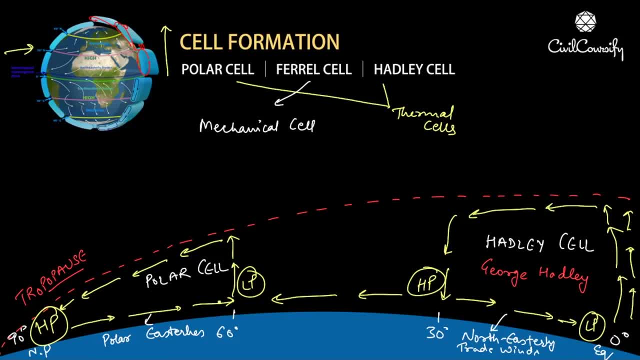 So wind will move in this direction And here it will converge with this wind and it will rise up And then, after going to the tropopause, it will move here And then it will converge after meeting this air mass coming from the equator. 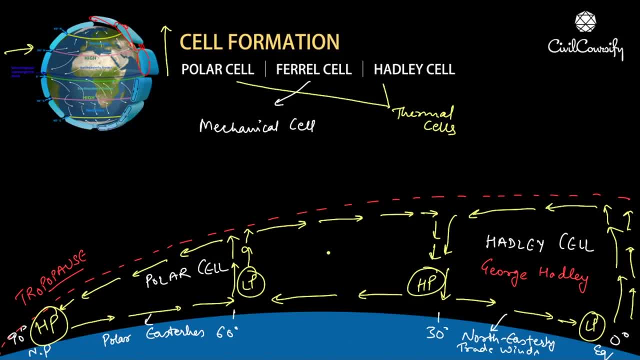 And finally, after subsiding, a cell will form. This cell is known as the ferrule cell. Now, this is known as the ferrule cell because this theory was given by William Ferrell, And this wind on the surface of the earth towards the poles is known as the westerlies. 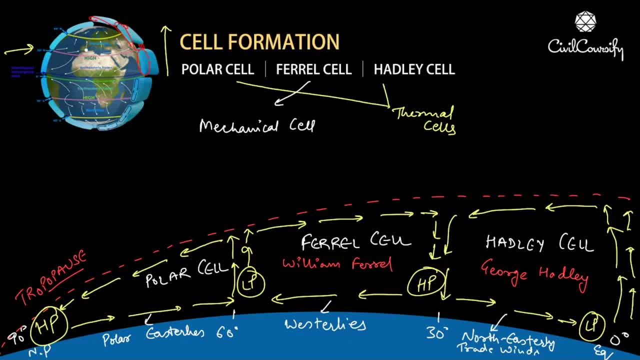 As you can see here, these are the westerlies in the temperate region. Now about the headly cell. you should know one thing about the headly cell: As the ITCZ shifts, this low pressure is formed on the ITCZ. We call it the equator for easy understanding. But this low pressure is actually formed on the ITCZ And the ITCZ keeps shifting throughout the year. That is why the headly cell also keeps shifting a little. Sometimes it will come a little to the north in the northern hemisphere. 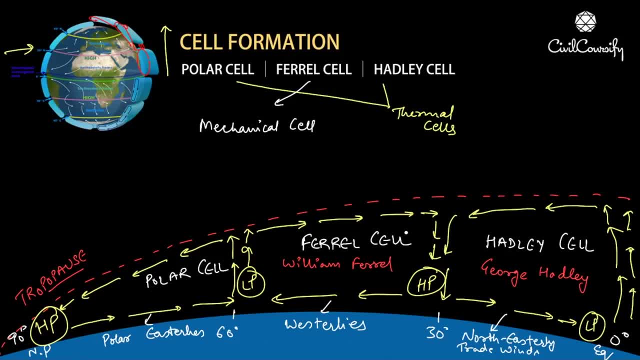 It can also shift a little towards the southern hemisphere Now, since the polar cell and the headly cell are thermal cells. they are very strong cells. Because they are strong, they do not change The north easterly trade winds, which are also known as the subtropical easterlies. and the polar easterlies. they are really strong winds And also there is not much terrain in the polar cell and the headly cell regions. Most of them are plains or deserts or cold deserts. Because of this, the winds here are very strong. 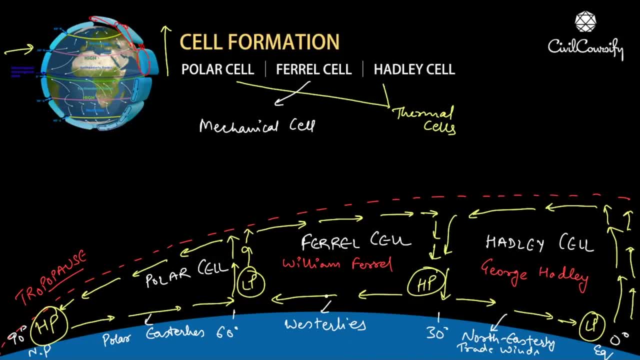 But the westerlies in the ferrule cell are very weak. That is why they are also called prevailing westerlies. They are weak because there is a lot of terrain. here There is a mountainous region on the earth. There is a lot of terrain.